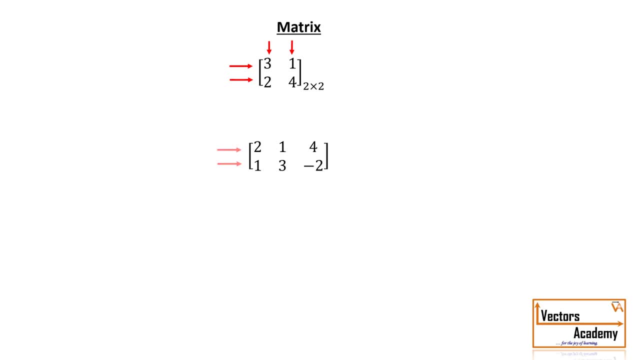 look at the second matrix. this matrix contains two rows, two horizontal rows and three vertical columns. Hence the order of this matrix is 2 into 3.. First we write the number of rows and then we write the number of columns. If you look at the third example, this matrix contains three rows and two columns. Hence the order is 3 into 2.. Now let us have a look at the different types of matrices. 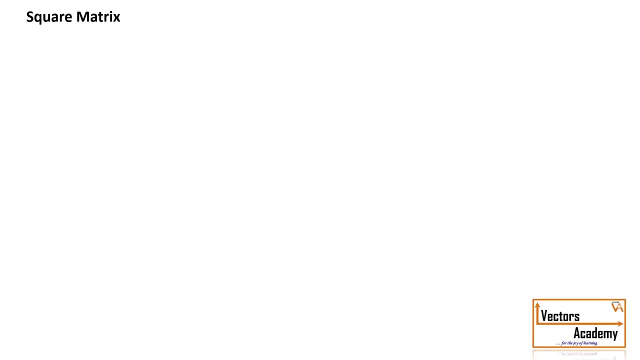 So the first, we have a square matrix. A square matrix is a matrix whose rows and columns are equal. Okay, the name itself suggests it's a square. all the sides should be equal, So we can have a 2 by 2 matrix or a 3 by 3 matrix, and so on. These are all square matrices. 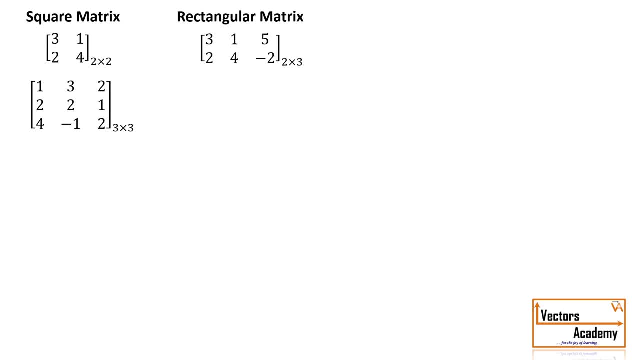 Next, we have a rectangular matrix whose rows and columns are not the same. Okay, they are different. This is a rectangular matrix. Then we have a diagonal matrix, a matrix whose elements, except the diagonals, are all zero, only the elements in the diagonal. 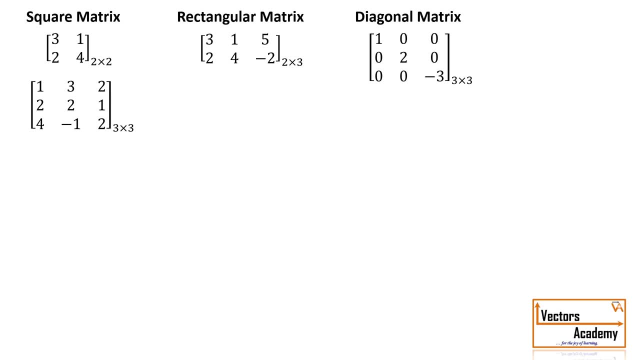 are non-zero elements. rest, all the elements are zero. a scalar matrix. a scalar matrix is in fact a diagonal matrix whose elements in the diagonal are same. okay, next we have a unit matrix, or the identity matrix. identity matrix is again a diagonal matrix whose elements in the diagonal 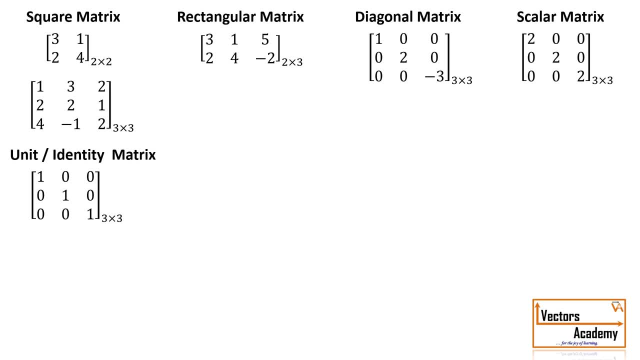 are in fact just one. hence you also call it as a unit matrix. okay, the next matrix is a zero matrix, whose all elements are zero, of course. next we have an upper triangular matrix. upper triangular matrix is a matrix whose elements above the diagonal are non-zero and below the diagonal 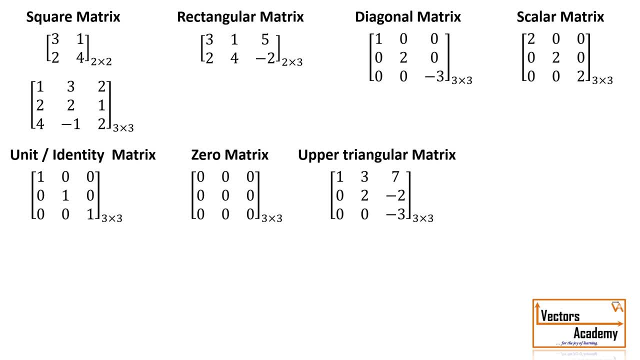 are zero. okay, the elements in the diagonal can be zero or non-zero, both. next, we have a lower triangular matrix whose elements below the diagonal are non-zero and above the diagonal the elements are zero. next, we have a symmetric matrix. now, symmetric matrix is a matrix whose element on both the sides- 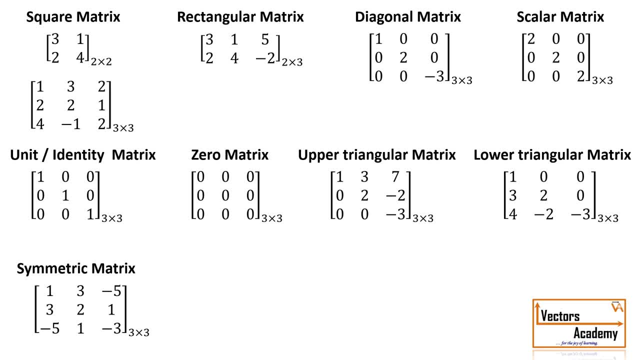 of diagonals are same. okay, you can see, the second element in the first row and in the first column is three. the third element, the first row and the first column is minus 5, and so on. Hence we can see the elements on both the. 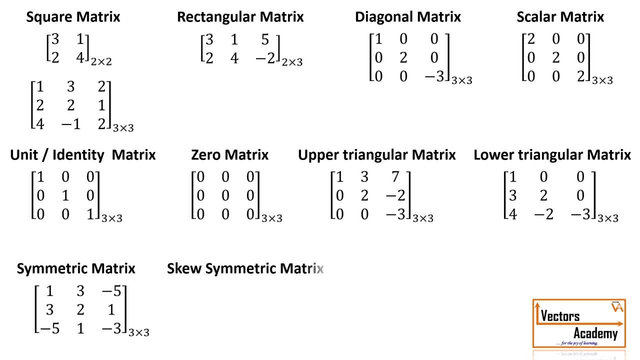 sides of diagonals are same, Hence it is called as a symmetric matrix, and the last one is a skew symmetric matrix, Now, a matrix whose diagonal elements are 0 and the elements on both the side of the diagonals are in fact same in magnitude but opposite in sign, So 3 and minus 3, minus 5. 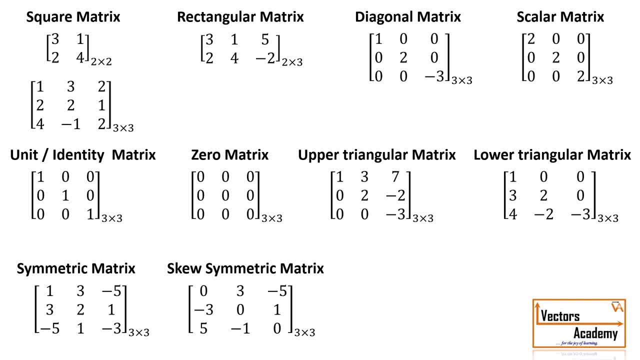 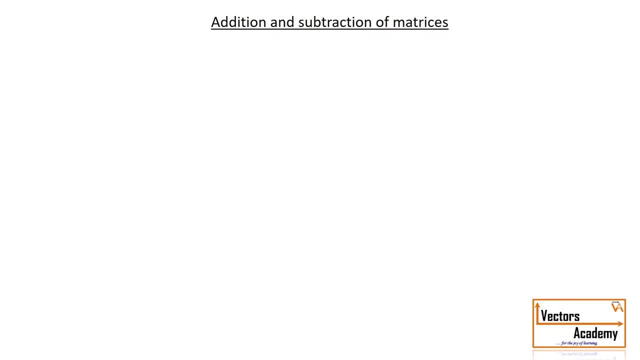 and 5, 1 and minus 1,. these are the same elements with opposite sign. So these are the different type of matrices. Now we will look how to add or subtract the matrices. Now the necessary condition to add or subtract the matrices is that their order should be same. The number of rows and 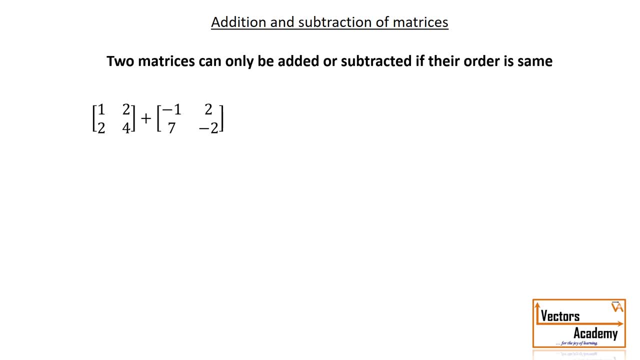 the number of columns. Both the matrices should be same. Now, if you look at these two matrices, we need to add them. So addition is quite simple. All we have to do is to add the first element of first matrix with the first element of second matrix, So that will give you 1 plus minus 1, that is 0. The second: 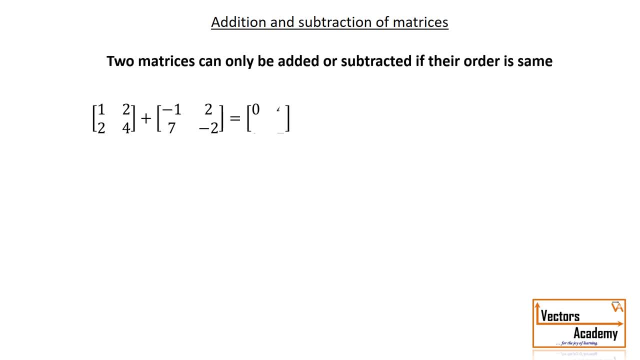 element of the first matrix with the second element of the second matrix, that is 2 plus 2,, will give you 4.. Then 2 plus 7 will give you 9, and 4 plus minus 2, that is 4,. 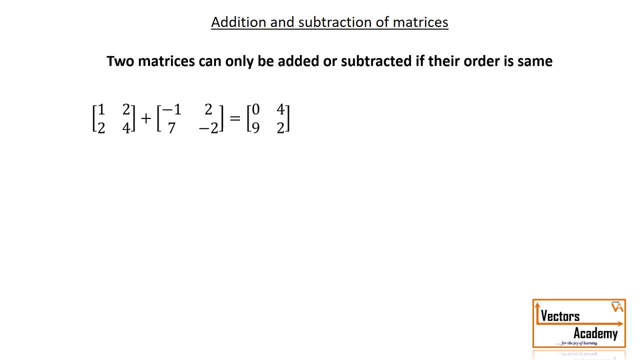 minus 2 will give you 2.. So it is quite simple. Let us have a look at another example. This time you have to subtract them, So 2 minus minus 3, that will be 2 plus 3, which will give you 5,. 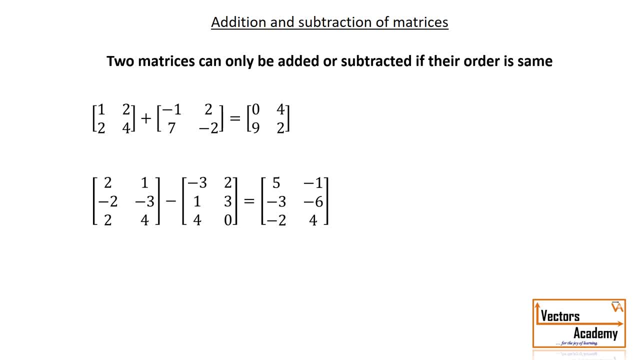 of course. Then 1 minus 2 will give you minus 1.. The element in the second row, this time minus 2 minus 1, will give you minus 3, and so on. We just subtract the corresponding elements in both. 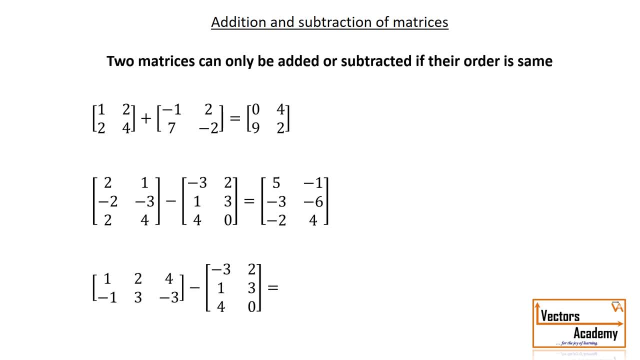 the matrices and we will get our answer Now. this time, the number of rows and number of columns in the first matrix and the second matrix is not same. Their order is different. The order of the first matrix is 2 by 3, whereas the order of the second matrix is 3 by 2.. Hence, these matrices cannot be.